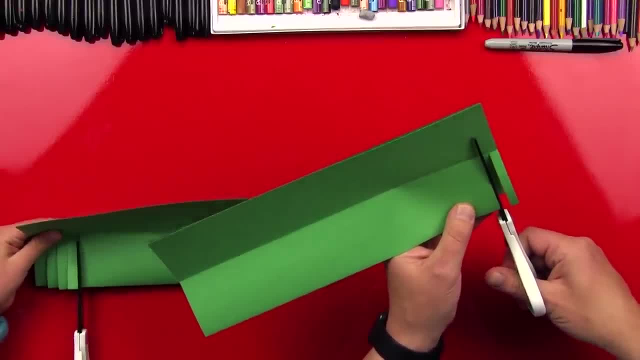 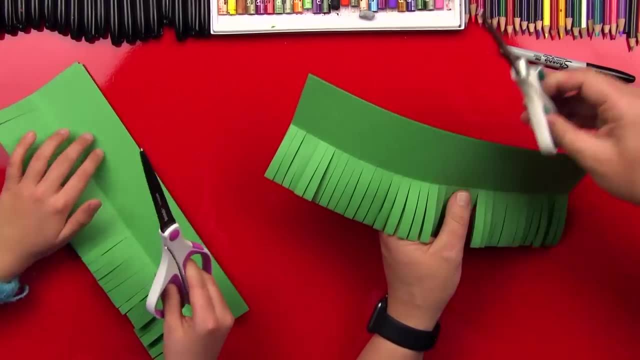 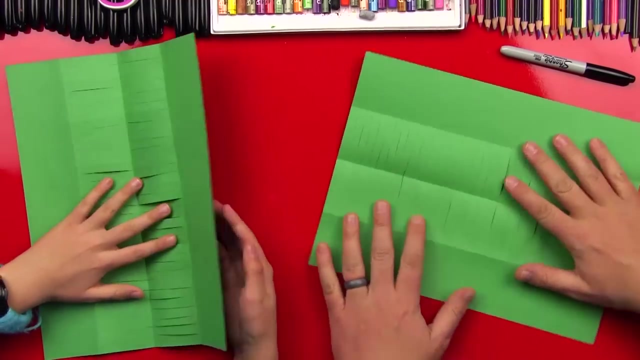 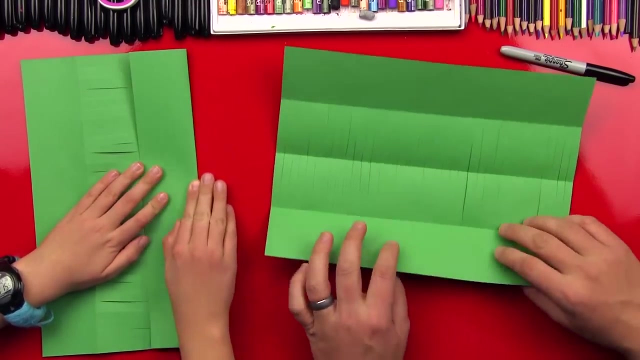 Okay, Right now. Awesome, are we done with our scissors? Yeah, at least for now. Yeah, Okay, Now what do we do now? We open it up, Okay, And then we, you can reverse any, Any one, it doesn't really matter which one. Okay, All right, so you can fold. 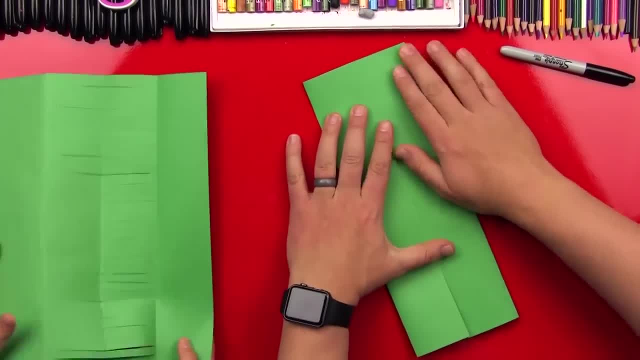 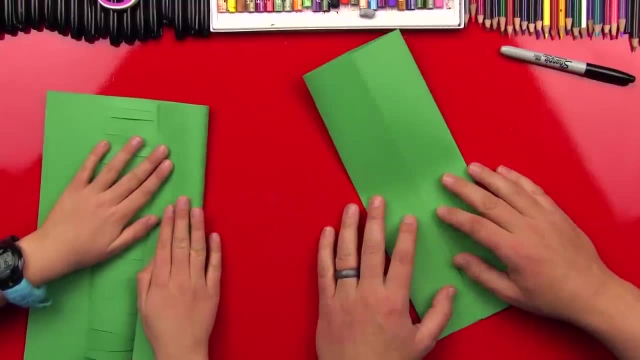 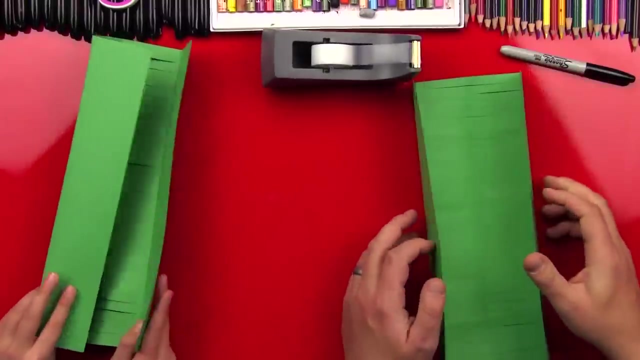 Fold them so that they fold in like this: Yeah, so you could reverse both of them, right? Yeah, okay, and then, and then that way they can fold in kind of like a book. cool, Now, what do we do? we need the tape. okay, I got the tape, it's right there now, but what do we do with it? 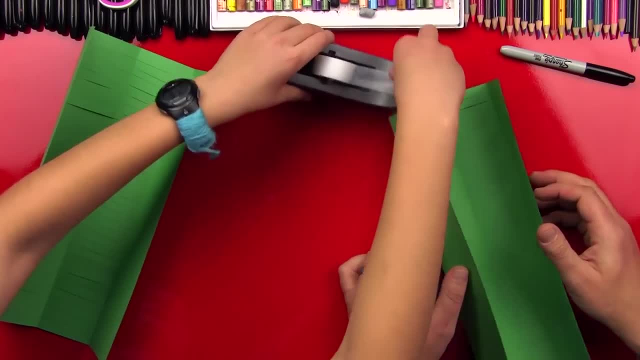 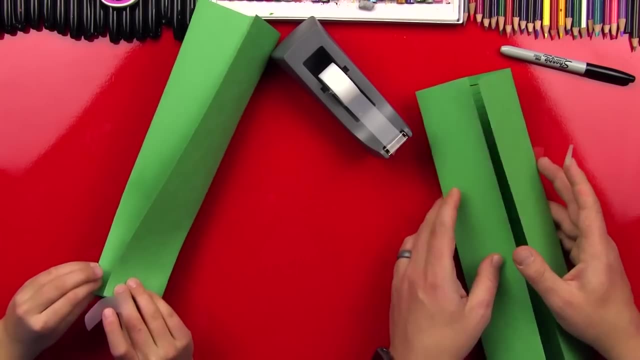 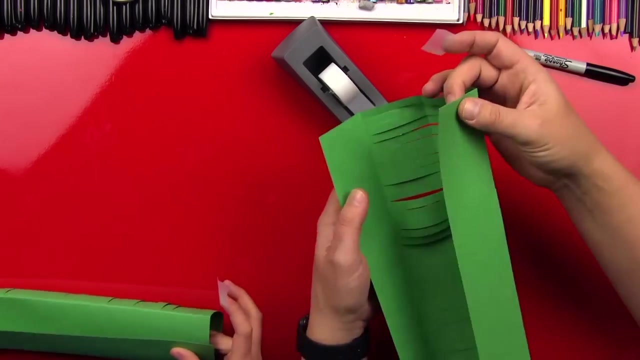 We, you get a piece- Yeah, it's a base or a piece of tape, Okay, And we could use glue for this, Yeah, okay, Okay, so it's like a triangle, like this, right, so this way, so you're over- you overlap these two and then 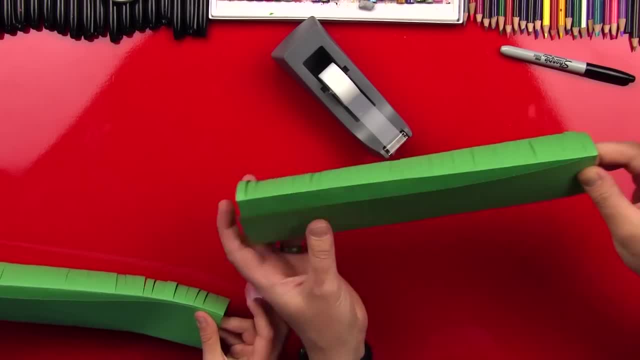 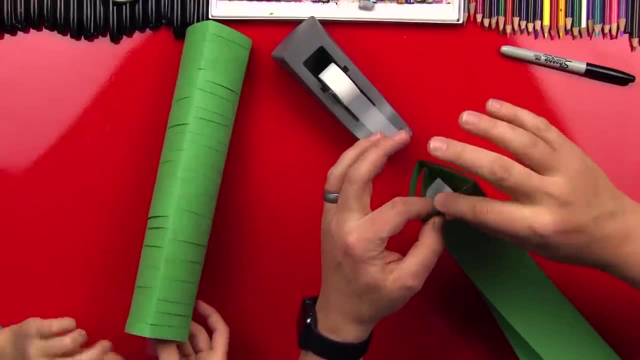 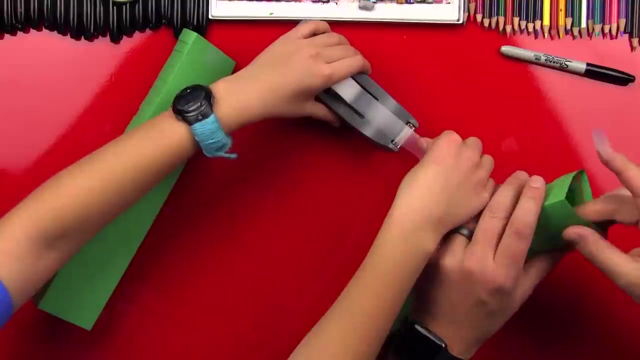 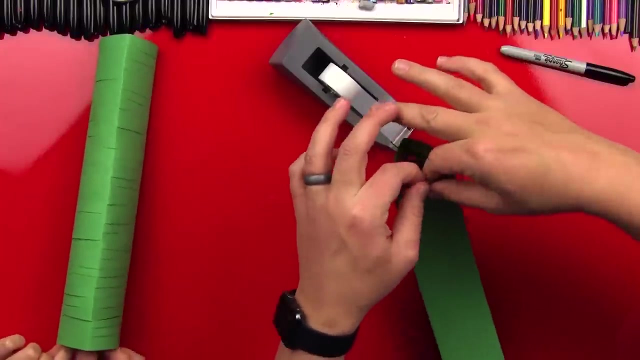 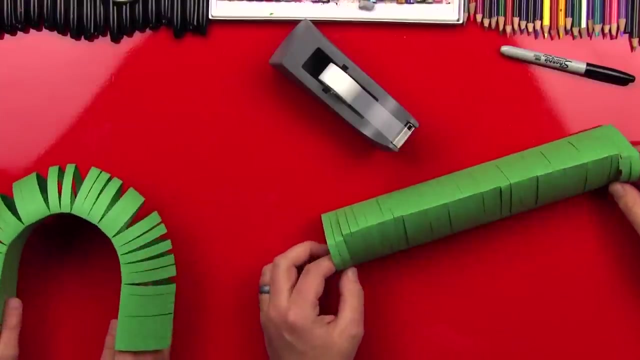 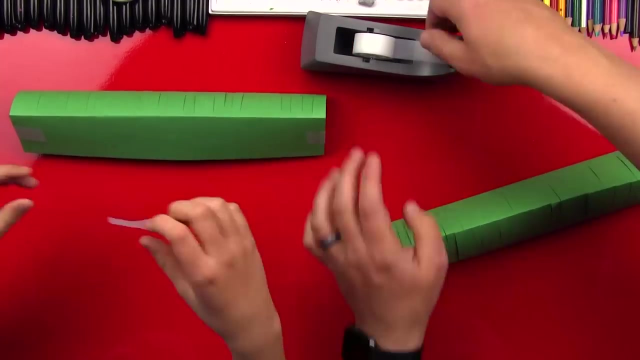 She makes a triangle like that: Okay, cool, the end together, the end case each and That. so I need another piece tape. okay, put it on there and then fold it inside. that way it stays. huh, yeah, cool, awesome. okay, okay, now what? okay, so next step: you need another piece of tape, another piece, okay, whoa, okay. 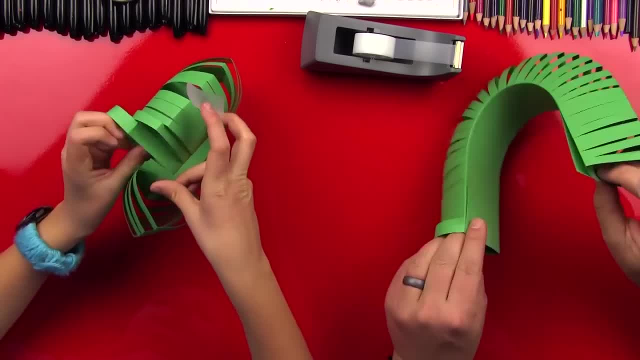 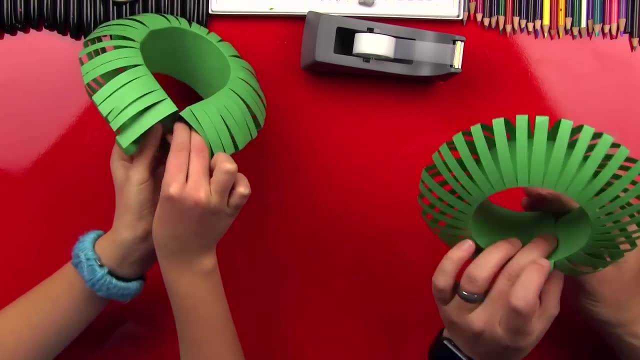 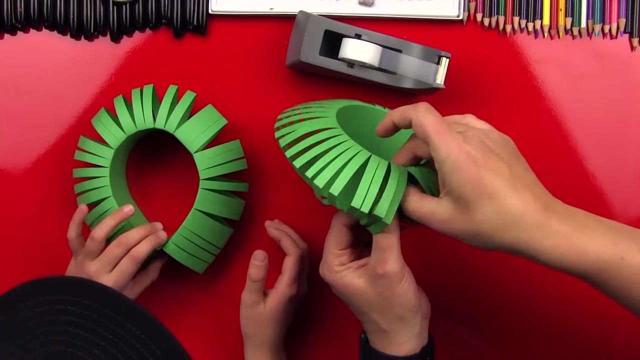 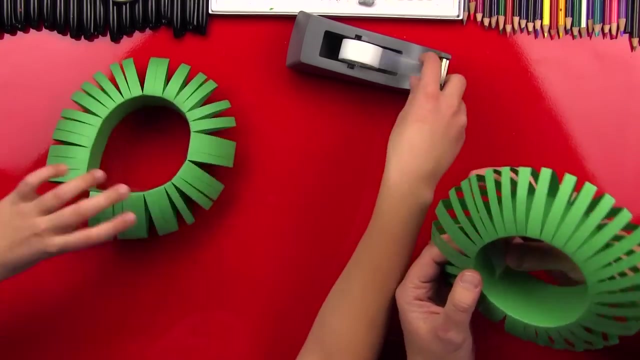 and then you, oh, I can see, look at that, it's already a wreath. and then you just take these two, okay. okay, so you put tape on the inside in here, and then you also put tape on the outside or in here. okay, they're all good ideas. huh, there's no bad ideas. 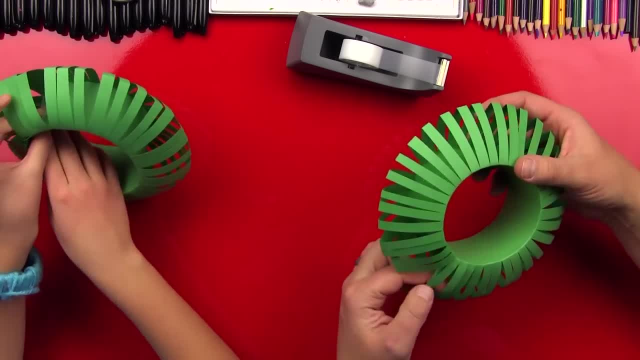 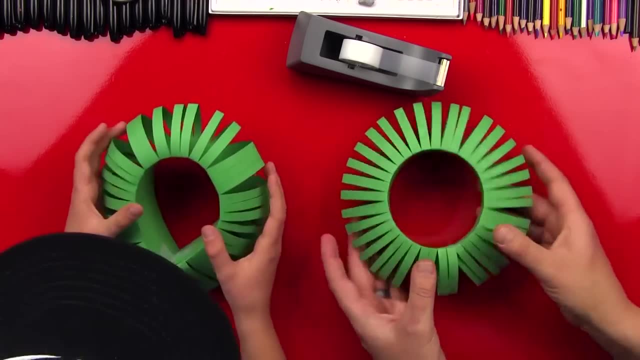 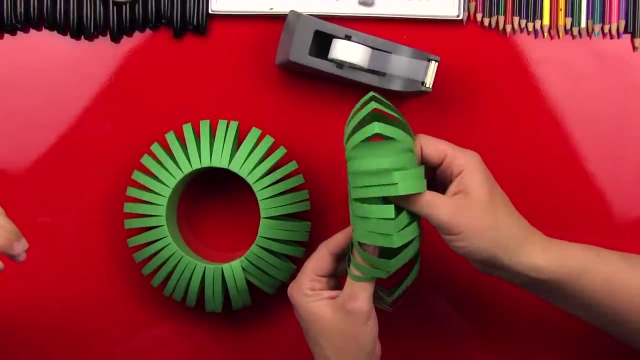 oh, dude, that looks so cool. I remember doing these when I was your age. yeah, yeah, that's awesome. it totally looks like a wreath. oh, that's okay. so we actually cut yours right, yeah, and then we're gonna overlap it, and I think that'll help it from doing a raindrop like that shape if you overlap it. 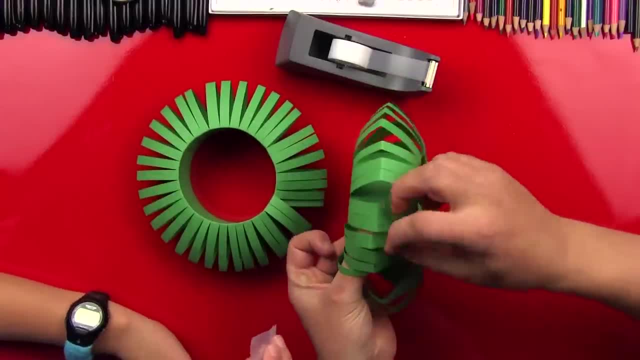 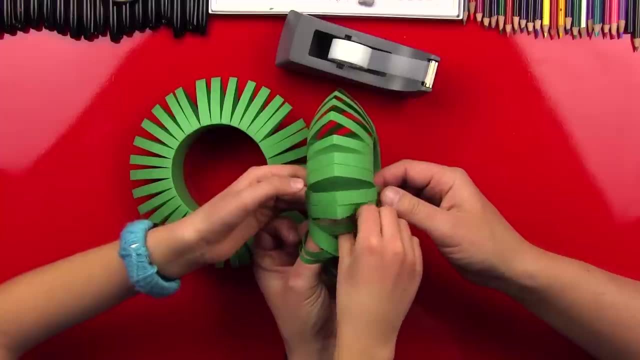 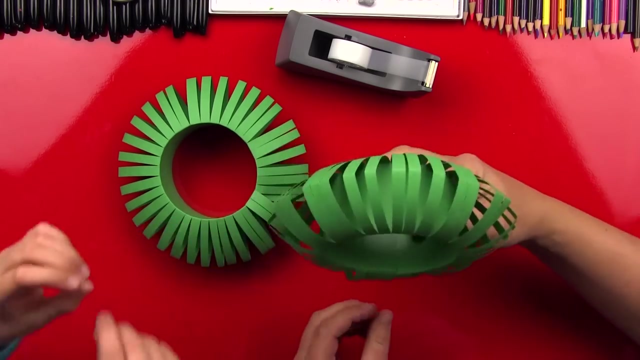 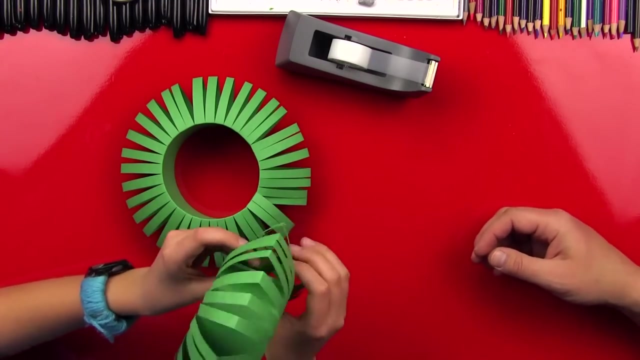 so we're gonna put tuck one side in slightly from the other one inside the other one and then take that thumbs in the way you could take it out. there we go, and then let's take the inside again there. nice, now they look really round. that's awesome. okay, now what, dude? we get the red piece. 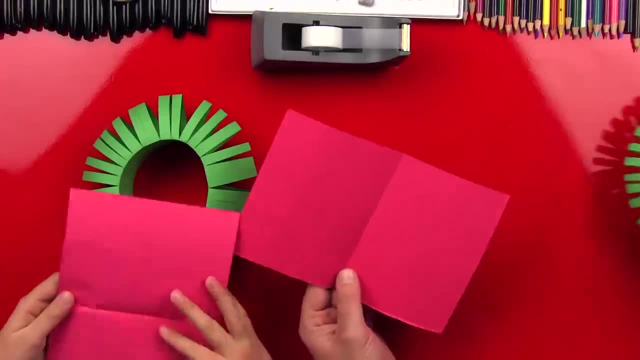 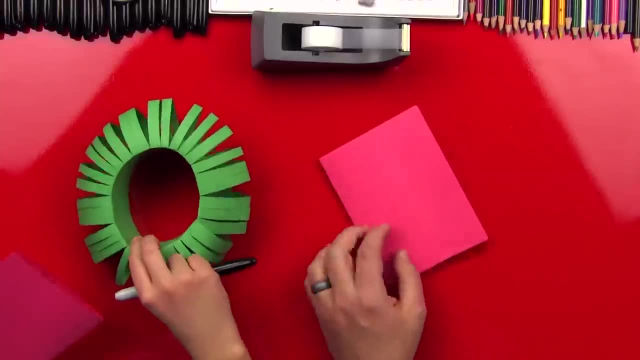 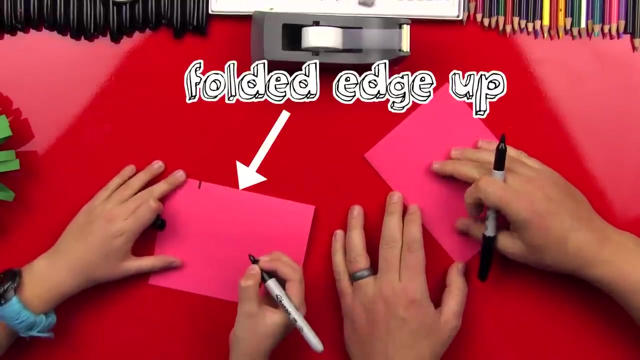 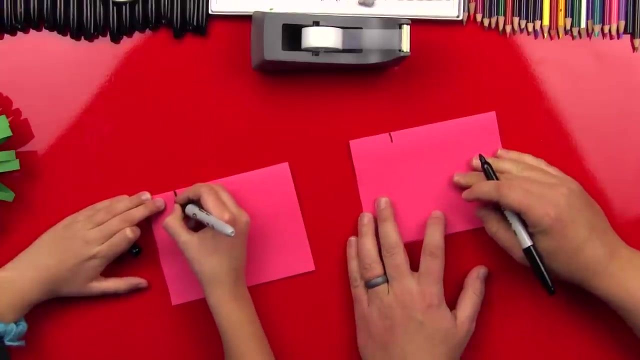 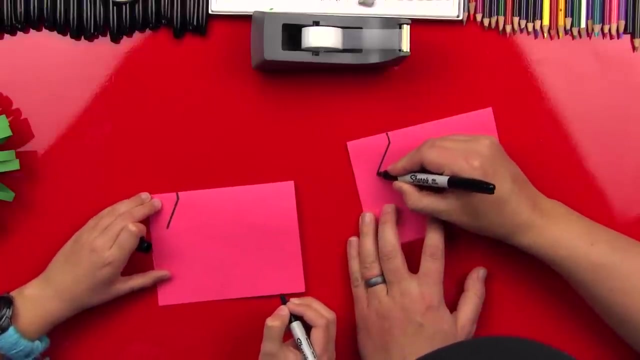 of paper. okay, oh yes, we did, and now we fold in half, you fold in half again, and then you could get your Sharpie. and then first you draw like a line out, okay, okay, like this line down, and then you, we're making the bow part. okay, so that's the knot, and then this is the bow, okay. 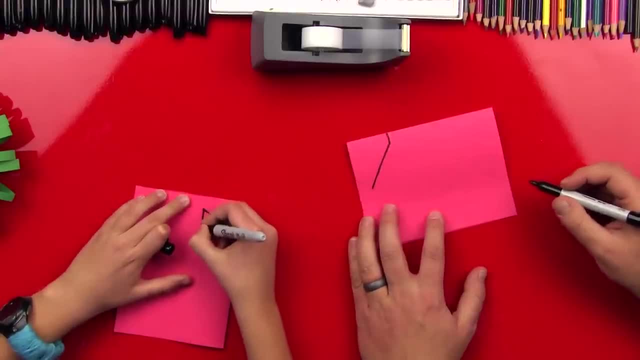 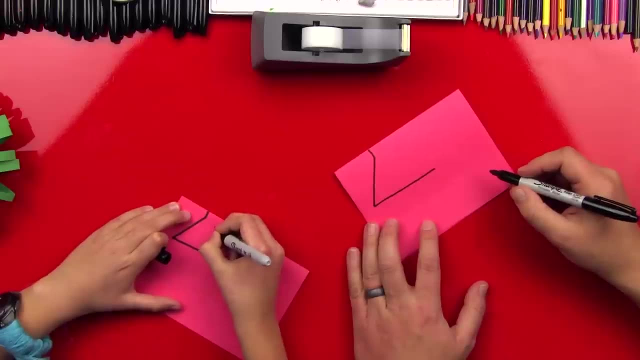 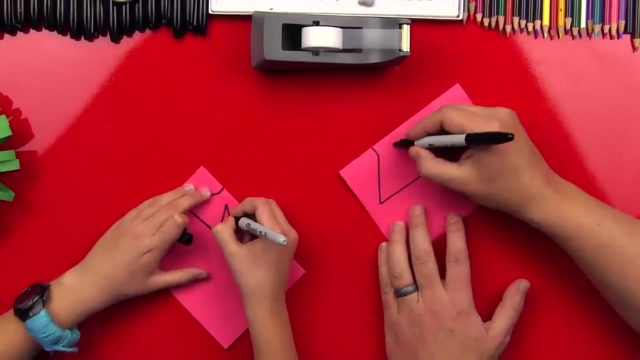 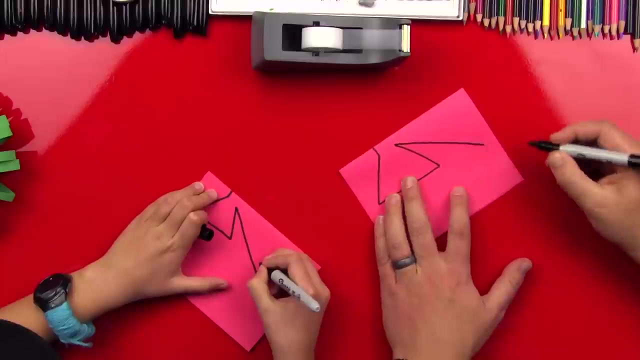 and then you go down, okay, and then you go back again, back up to the same kind of the same spot, okay, and then you go out a little longer. oh, that's the bottom part of the bow. huh, okay, i'm gonna do a v. whoa cool. 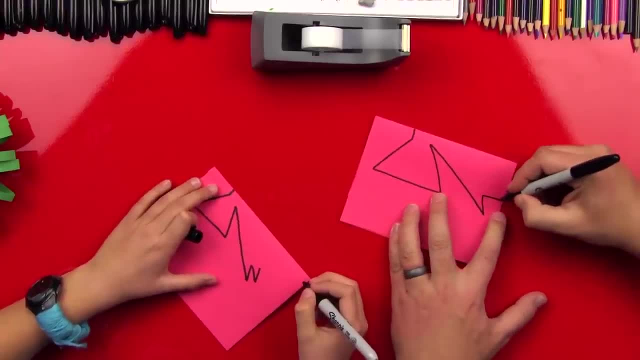 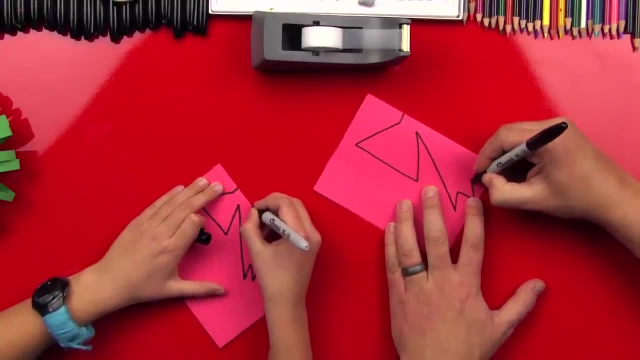 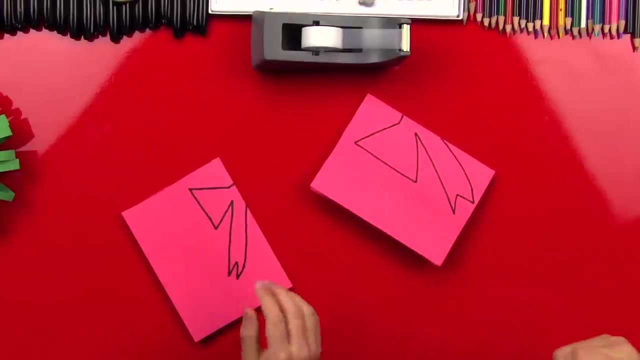 okay, w, uh, w and back up, okay. and then you go up and go up and connect it. no, you just keep them going. connect it to the outset, to here: yeah, cool, awesome, now what? and then you cut it. and then you cut it. okay, i got my scissors, it's mine, right there. 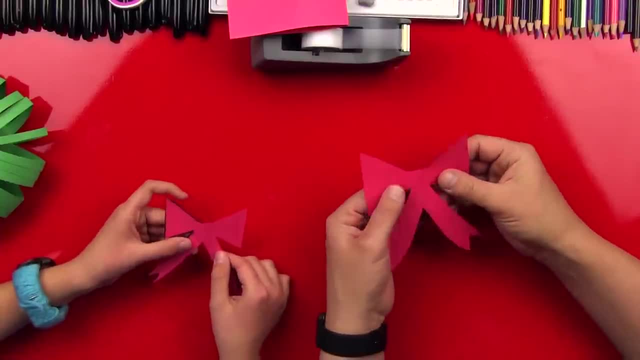 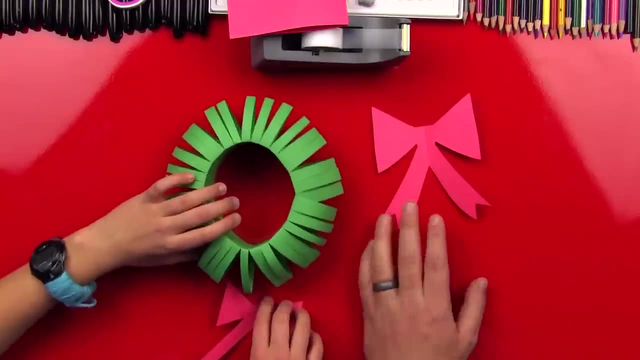 all right, i got it out. okay, oh, and then we can open it. that looks awesome. mm-hmm, that looks really cool. that's a simple way to do a bow. yeah, okay, next. what's next? you bring your wreath back. okay, wreaths back, and then you get your tape. 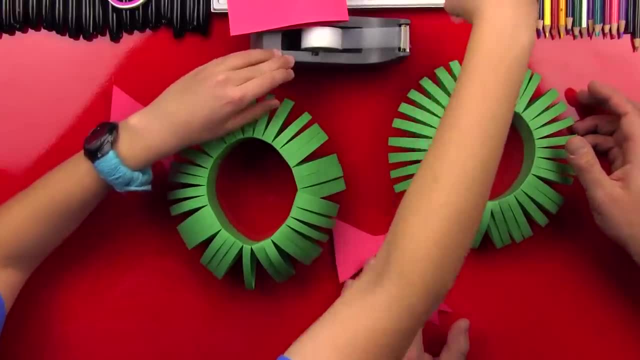 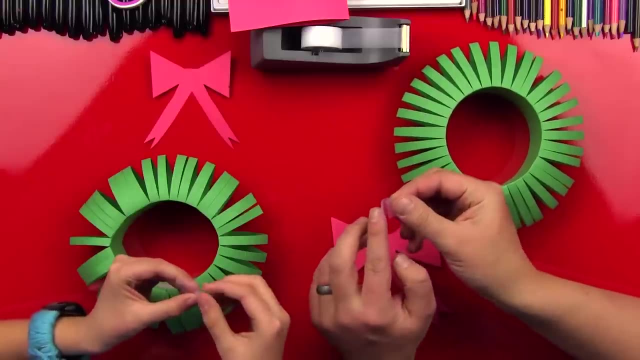 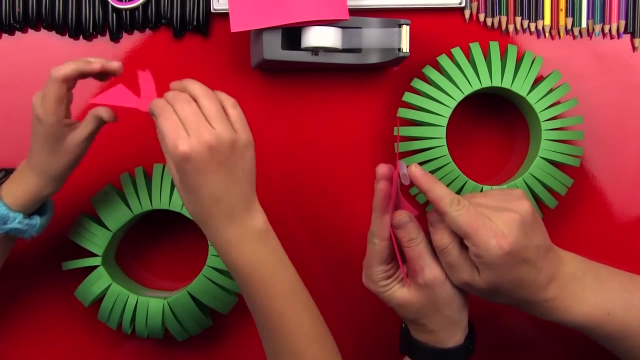 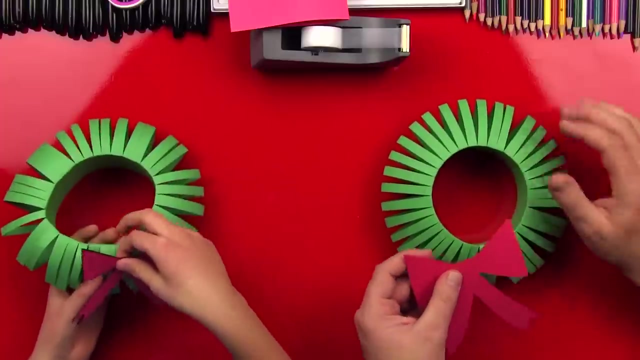 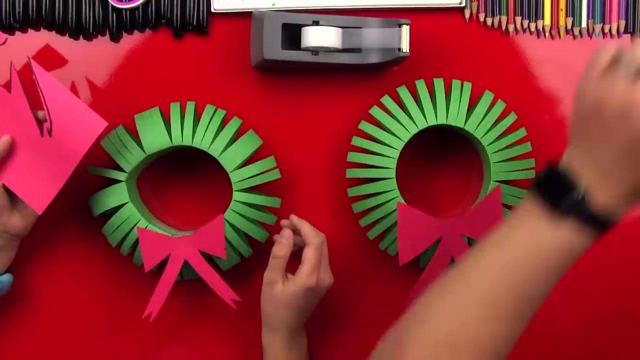 okay, piece, okay, and then you just do, you flip this around so you get a little tape roll, okay, and then you put it on the spot where you taped, oh, where they came together. yeah, put that at the bottom, okay, um, and then you bring the red paper back. okay, i got more red paper and then 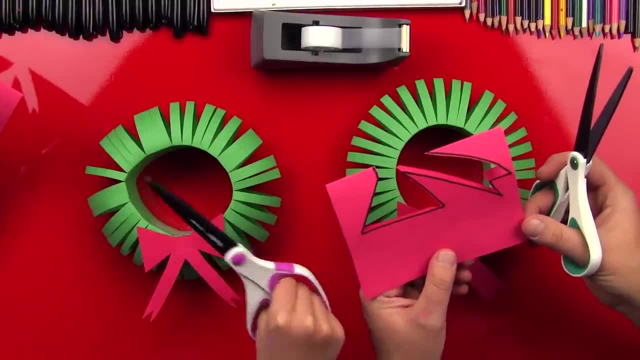 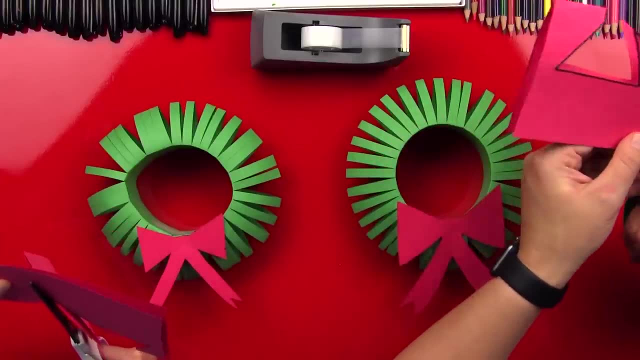 you can leave it folded for like more, for more. okay, what are we making next? the berries, cool, okay. so what are we gonna cut out the circles? okay, now, if we leave it folded, then we can cut two berries at the same time. make more, cut two berries at the same time. 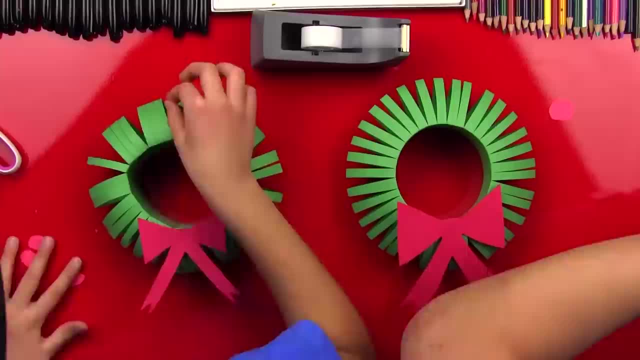 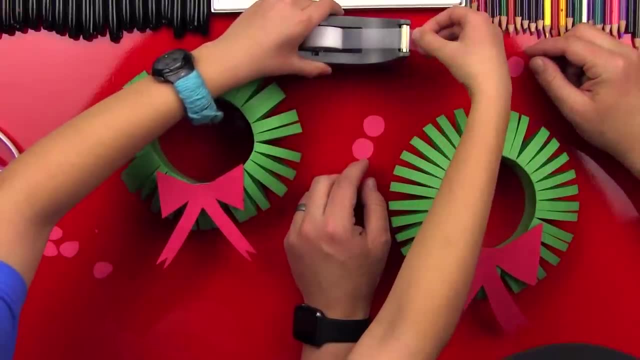 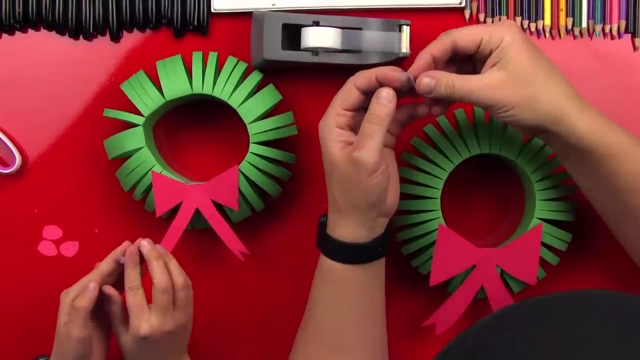 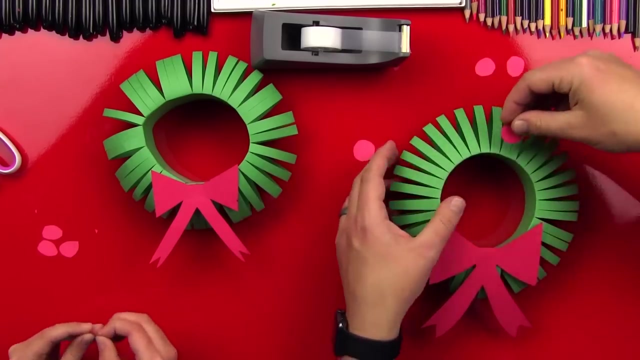 same time. all right, yeah, okay, i got my berries cut out. okay. next you get a little piece of tape, not really big, and then do the same thing. this might be where- yeah, if, if our friends wanted to use glue, it might work a little. yeah, it might be easier to hide the tape, right, and you just stick them on. yeah. 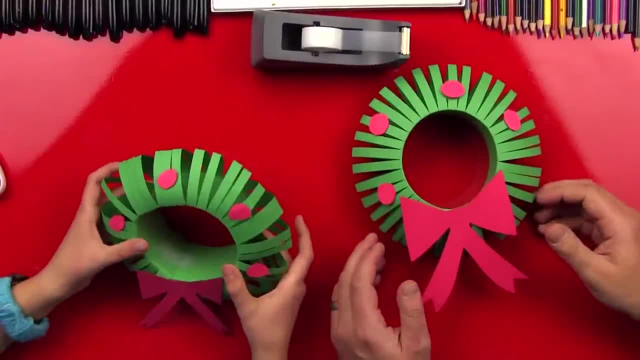 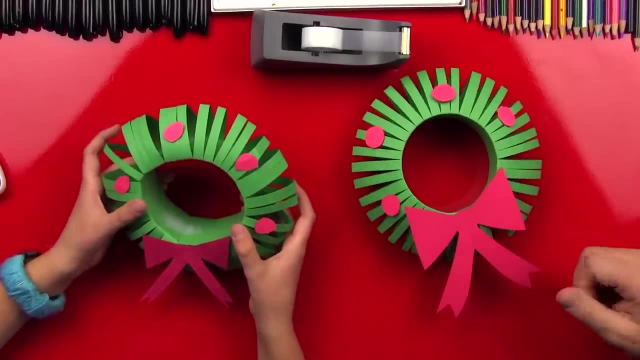 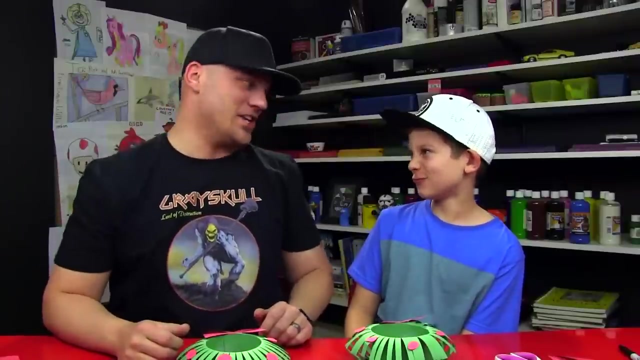 check them out. yeah, i think you're the best teacher on the planet. you did such a good job at teaching me how to do this. i totally forgot how to make them and now i feel like a kid again. give me five, yeah. yeah, did you have fun? yes, good, we hope you guys had a lot of fun making a wreath. 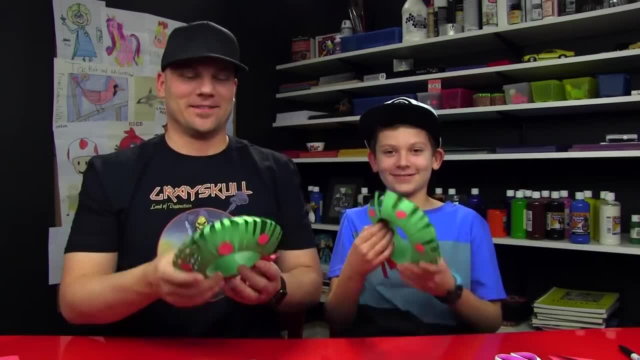 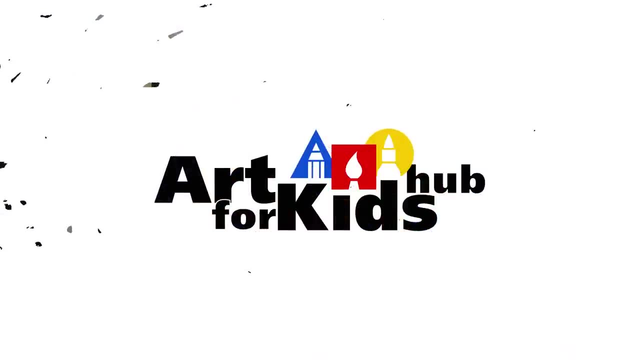